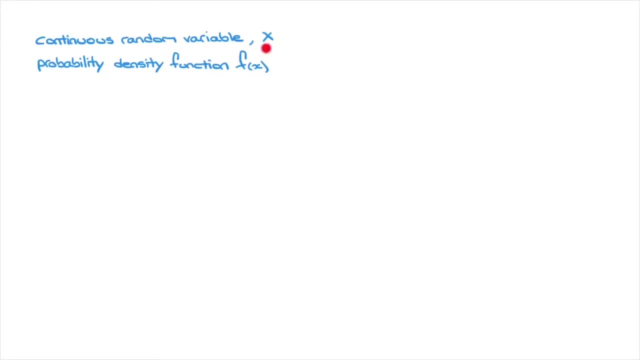 dealing with a continuous random variable called capital X and that it has a probability density function, a pdf f of x. Now the formula for calculating the mean is the following: We write mu, which is the greek equivalent of our letter. m equals to the integral from negative infinity. 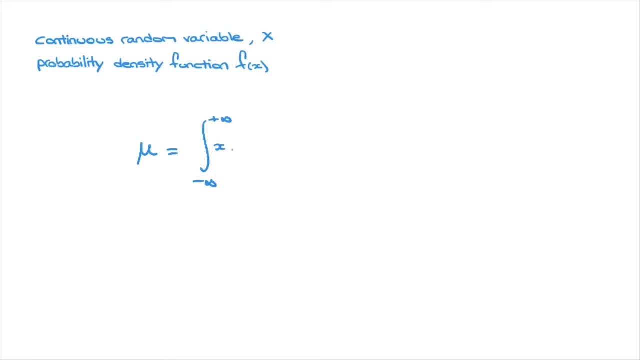 to positive infinity of x times f of x, where f of x is the probability density function of the continuous random variable. As I said previously, the mean is the probability density function of the continuous random variable. The mean is also called the expected value, and this formula can therefore also be written as: 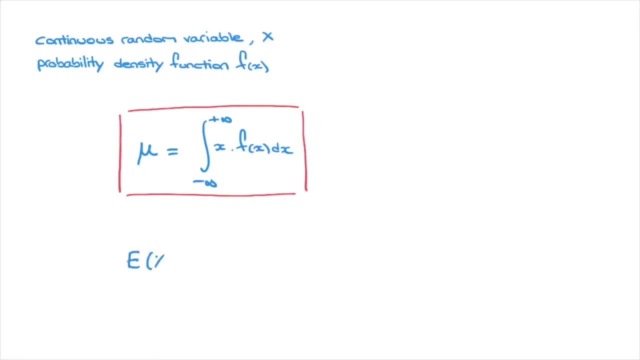 follows: Capital E of capital X equals to the integral, from negative infinity to positive infinity, of x times f of x. To be clear, both of these formula are exactly the same. The only distinction is the terminology. In the first we're referring to the mean value and in the second 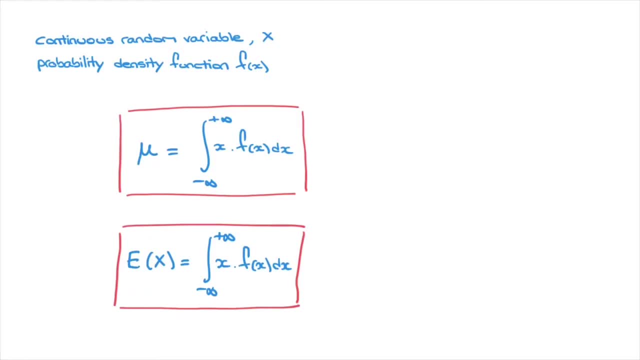 we're referring to the expected value. Both things mean exactly the same thing. Okay, now that we've seen the formula, let's go ahead and learn how to use it with a worked example. Here's an example. We're told that the time in seconds it. 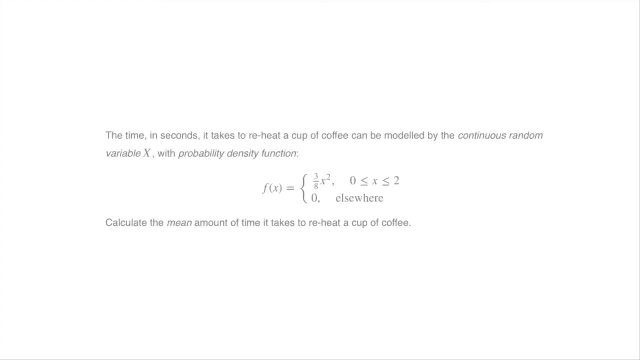 takes to reheat a cup of coffee, can be modeled by the continuous random variable, capital X, with probability density function f of x, which equals to the piecewise function defined as 3, 8 of x squared for all of x contained between 0 and 2, and it's equal to 0 elsewhere, And we're asked to calculate the mean. 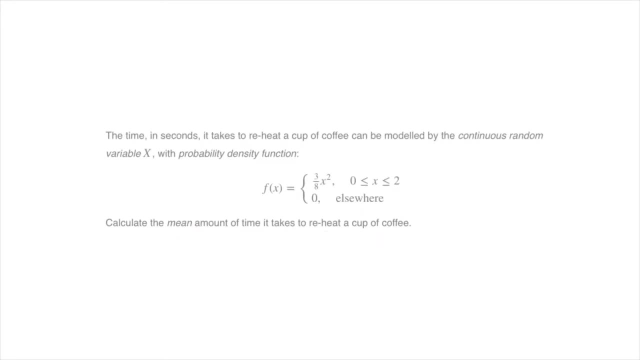 amount of time it takes to reheat a cup of coffee. In other words, we need to calculate the mean of this continuous, random variable, capital X. I'll start by moving this question to the side a little bit. There we go. Now let's get started By definition. as we've just seen, the mean is mu, which equals to: 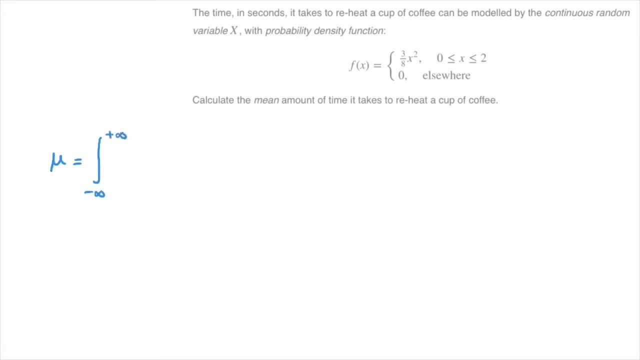 the integral from negative infinity to positive infinity of x times f of x squared. Now let's get started By definition, as we've just seen, the mean is mu, which equals to the integral from negative infinity to positive infinity of x times f of x. 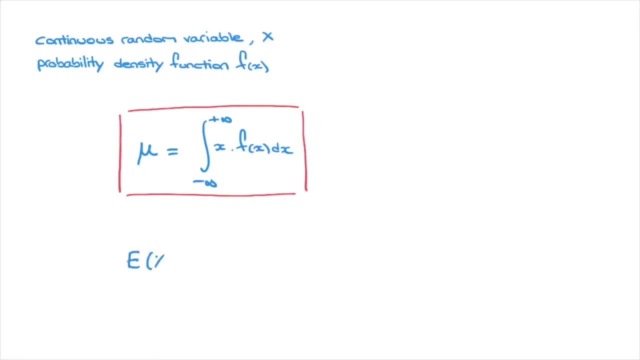 follows: Capital E of capital X equals to the integral, from negative infinity to positive infinity, of x times f of x. To be clear, both of these formula are exactly the same. The only distinction is the terminology. In the first we're referring to the mean value and in the second 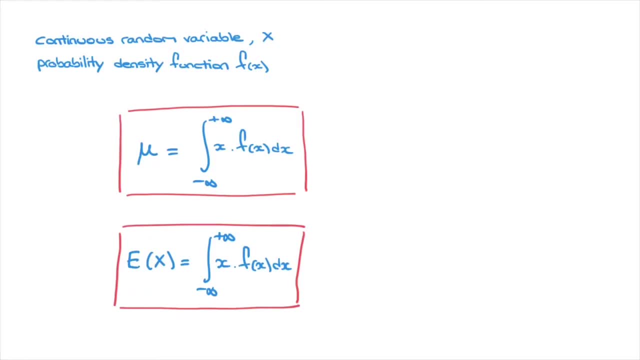 we're referring to the expected value. Both things mean exactly the same thing. Okay, now that we've seen the formula, let's go ahead and learn how to use it with a worked example. Here's an example. We're told that the time in seconds. 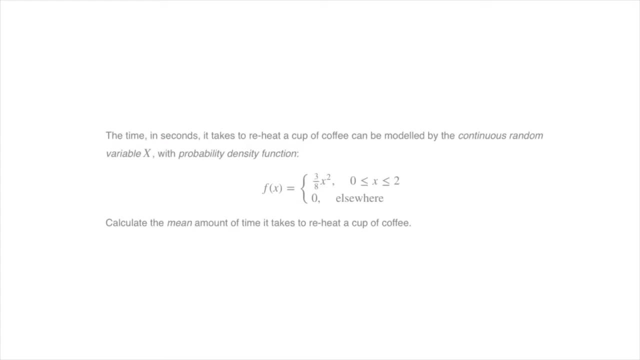 it takes to reheat a cup of coffee can be modeled by the continuous random variable capital X, with probability density function f of x, which equals to the piecewise function defined as three-eighths of x squared, All x contained between zero and two, and it's equal to zero elsewhere. And we're asked to: 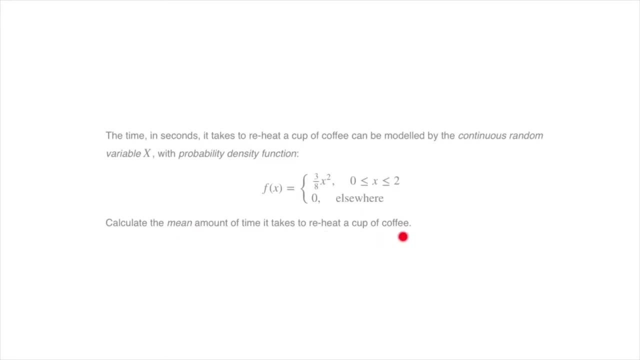 calculate the mean amount of time it takes to reheat a cup of coffee. In other words, we need to calculate the mean of this continuous random variable, capital X. I'll start by moving this question to the side a little bit. There we go. Now let's get started By definition, as we've just 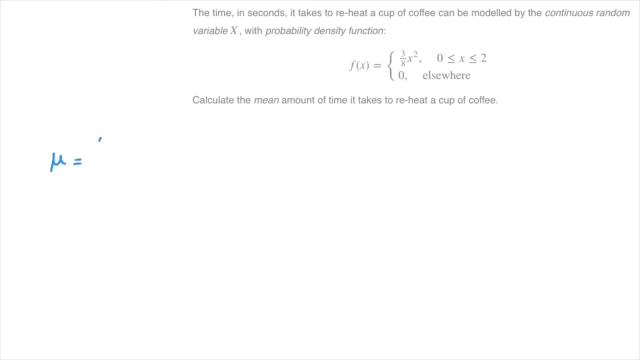 seen, the mean is mu, which equals to the integral, from negative infinity to positive infinity, Of x times f of x, where f of x is the probability density function. Now, looking at the probability density function that we're given in the question, we can see that for all x outside of the interval, 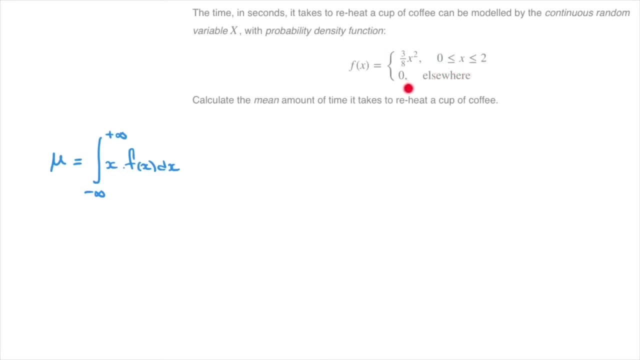 zero to two, the function is equal to zero. Consequently, this integral turns into the following: It's equal to the definite integral, from zero to two, of f of x squared, And we're given x times three-eighths of x squared. Multiplying these two x's together and taking the 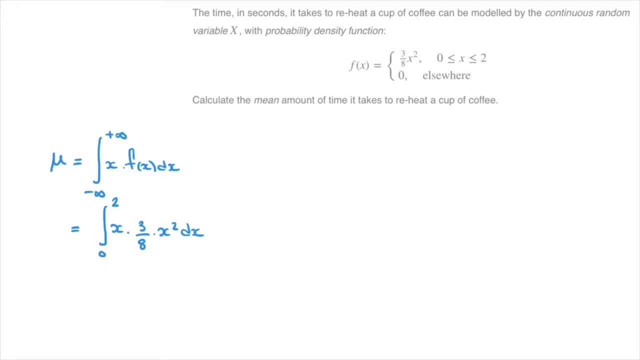 three-eighths outside of the integral. we can write that this equals to three over eight times the definite integral. from zero to two of x cubed, That's equal to three over eight times in square brackets x to the power of four over four, with lower limit zero and upper limit. 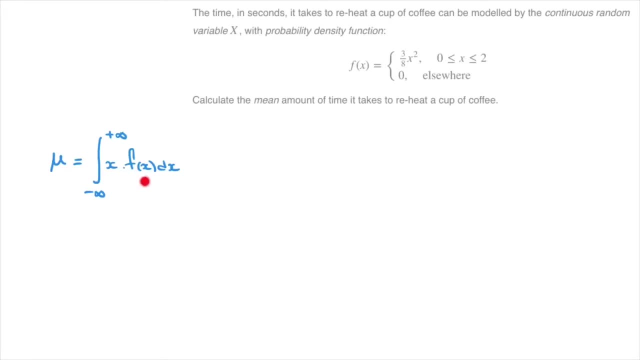 Where f of x is the probability density function. Now, looking at the probability density function that we're given in the question, we can see that for all x outside of the interval 0 to 2, the function is equal to 0. Consequently, this integral turns into the following: It's equal to the definite integral. 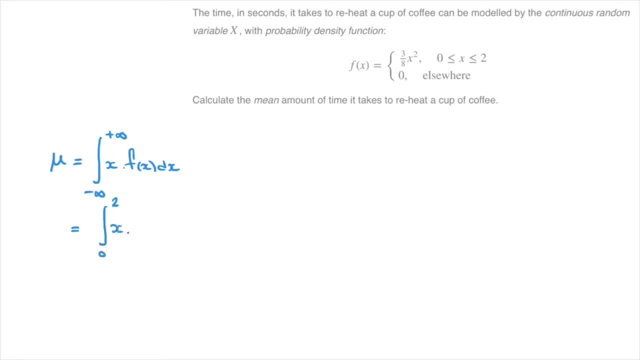 from 0 to 2 of x squared squared. squared x times 3 8ths of x squared. Multiplying these two x's together and taking the 3 8ths outside of the integral, we can write that this equals to 3 over 8 times the definite integral. from 0 to 2 of x cubed. 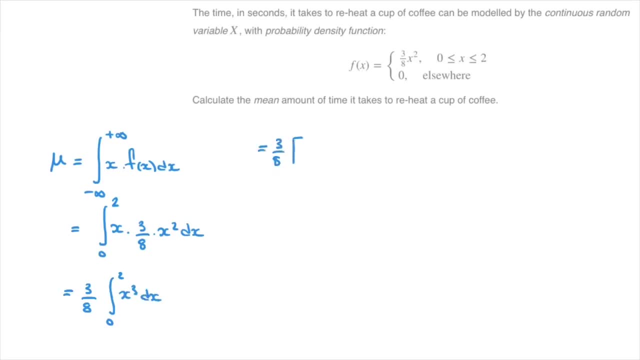 That's equal to 3 over 8 times in square brackets, x, to the power of 4 over 4, with lower limit 0 and upper limit 2.. That's equal to 3 over 8 times, in square brackets, x to the power of 4 over 4, with lower limit 0 and upper limit 2.. 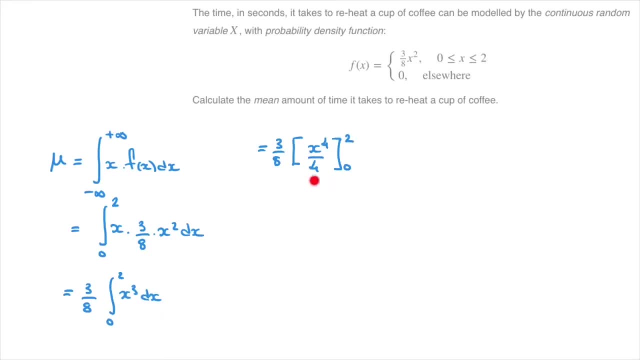 And to make life easier, I like to take this factor of a quarter outside of these square brackets. So this would equal to 3 over 8 times 1 over 4 times in square brackets, x to the power of 4, with lower limit 0 and upper limit 2. That's equal to 3 over 32 times in square brackets. 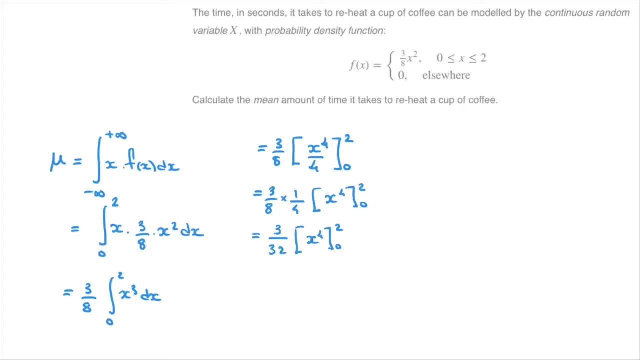 x to the power of 4, with lower limit 0 and upper limit 2.. This equals to 3 over 32 times 2 to the power of 4, minus 0 to the power of 4, and that's equal to 3 over 32 times in square. 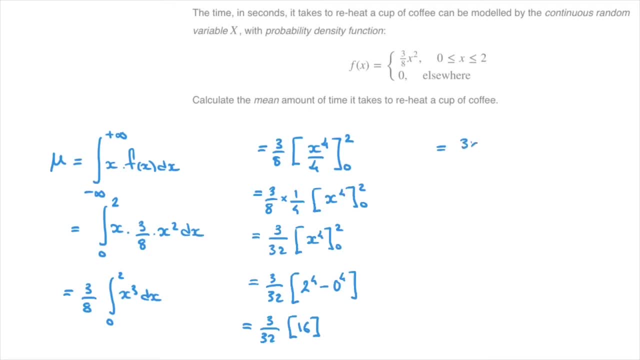 brackets 16, which equals to 3 times 16, over 32, which is 2 times 16.. Finally, the mean mu is equal to 3 over 2, which is a decimal, is equal to 1.5.. And that's how to calculate the mean of a continuous. 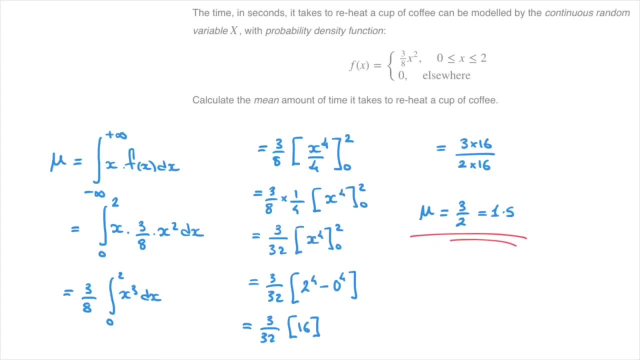 random variable. Now, this mean tells us what we could expect the average or mean value of the continuous random variable to be after a sufficiently large number of trials. So, given this scenario- the scenario in which we're reheating a cup of coffee- what this tells us is that if we were 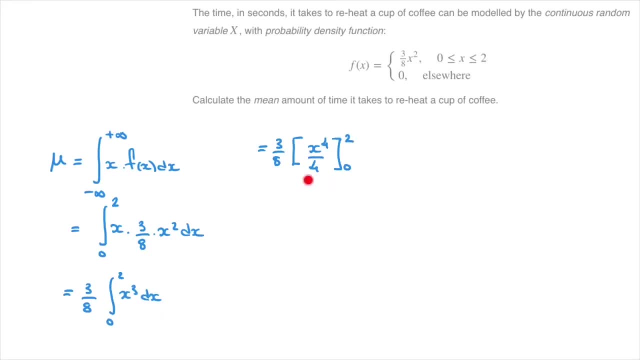 two. And to make life easier, I like to take this factor of a quarter outside of these square brackets. So this would equal to three over eight times one over four times in square brackets, x to the power of four, with lower limit zero and upper limit two, That's equal to three over thirty-two. 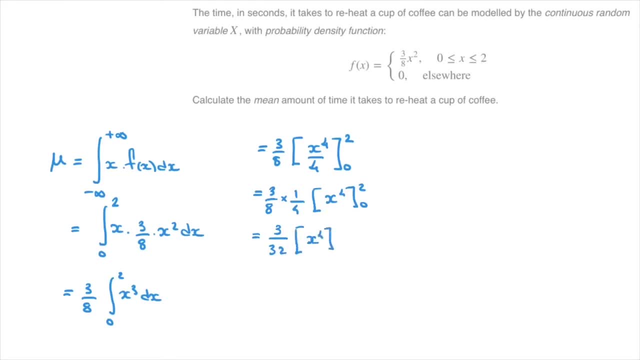 times, in square brackets, x to the power of four, with lower limit zero and upper limit two. This equals to three over thirty-two Times two to the power of four, minus zero to the power of four, And that's equal to three over thirty-two. 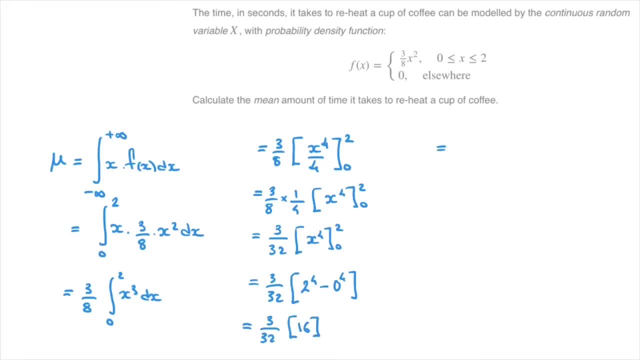 times, in square brackets, sixteen, Which equals to three times sixteen over thirty-two, which is two times sixteen. Finally, the mean mu is equal to three over two, Which as a decimal, is equal to one point five. And that's how to calculate the mean of a continuous random variable. 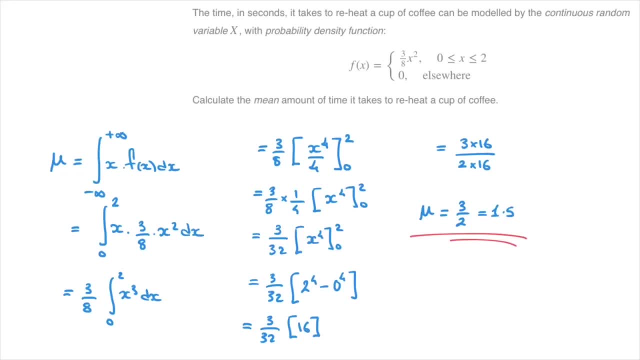 Now, this mean tells us what we could expect the average or mean value of the continuous random variable to be after a sufficiently large number of trials. So, given this scenario- the scenario in which we're reheating a cup of coffee- what this tells us is that, if we were to make a note of the 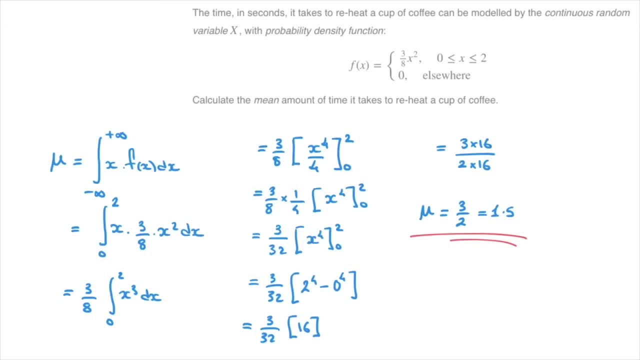 time that it takes to reheat a cup of coffee a hundred times, or a thousand times, or even a million times, then the average of all the times that we'll have written down will tend to towards 1.5 seconds. And that's what the mean tells us. And that's it for this tutorial. 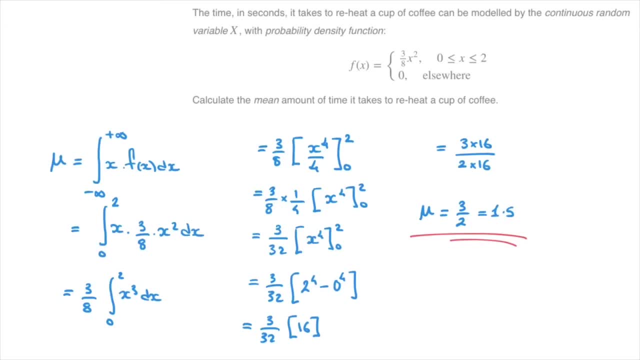 to make a note of the time that it takes to reheat a cup of coffee a hundred times or a thousand times or even a million times, then the average of all the times that we'll have written down will be 1.5 seconds, And that's what the mean tells us. And that's it for this tutorial. 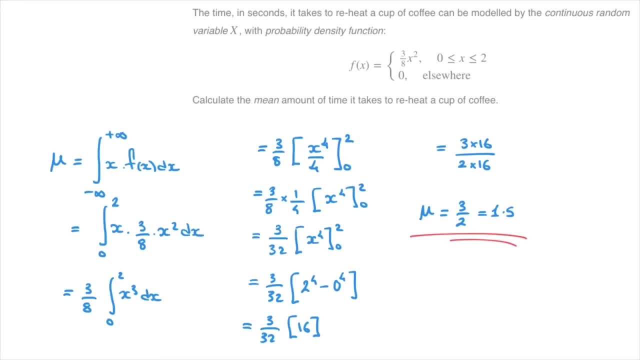 There we go everyone. I really hope that helped and if it did, please hit like on this video and even subscribe to our channel, because that really does help us. I'll see you soon. 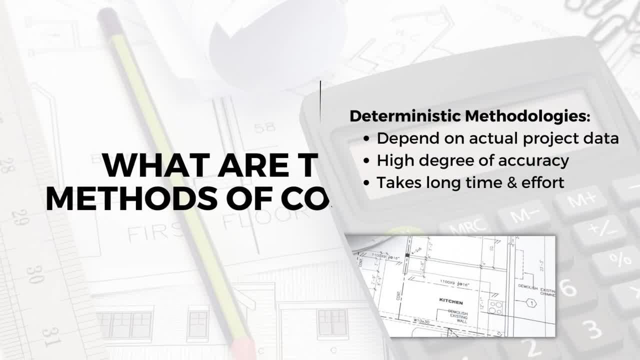 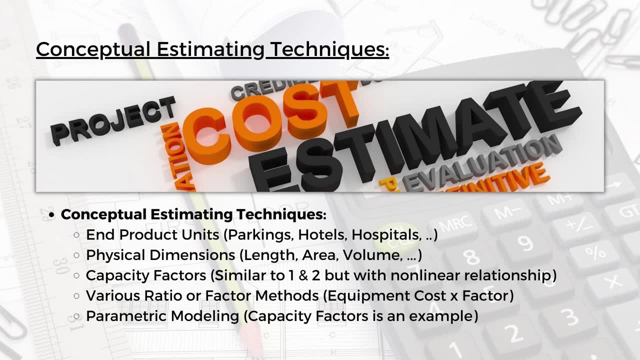 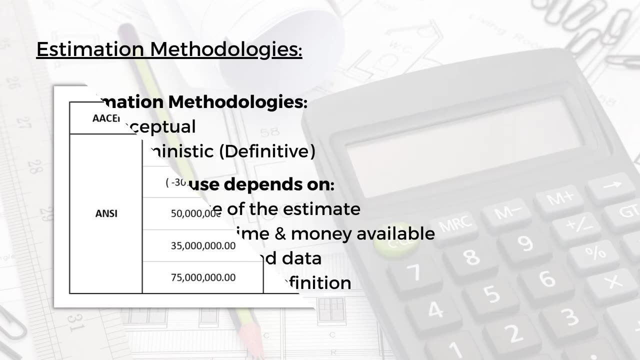 In this video, I'll elaborate the common methods of cost estimation, including the difference between conceptual and deterministic methodologies, the level of effort required and when to use each of them. The information presented in this video is taken from Skills and Knowledge of Cost Engineering, which is a book produced by the AACEI and it's 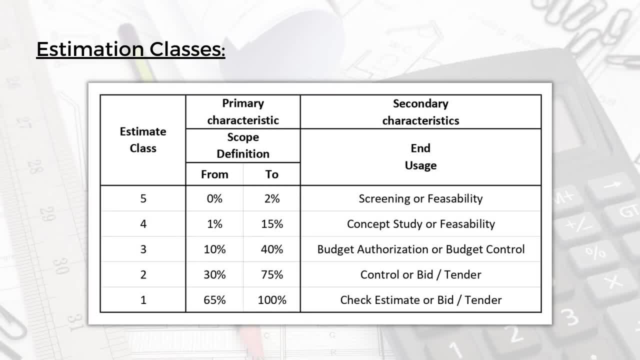 a very reliable source of information. So, starting with the estimation classes, we have five classes of estimate class five, four, three, two, one. And actually what differentiates these classes from each other? We have two things: We have the primary characteristics and we have the secondary. 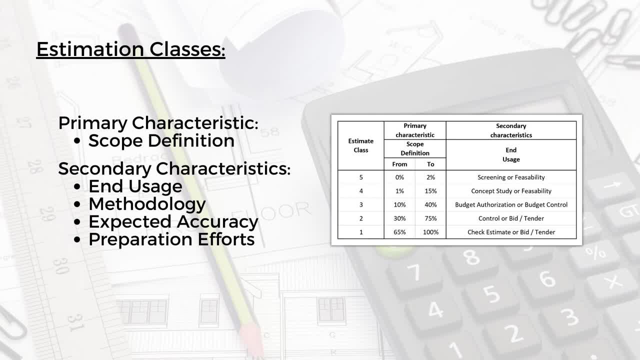 characteristics, which means what makes a class three, for example, a class three. It depends on some primary characteristics and some secondary characteristics, And the primary one is the scope definition. This is the most important characteristic that differentiates these estimate classes. And we have also secondary characteristics, which are the NDEs. 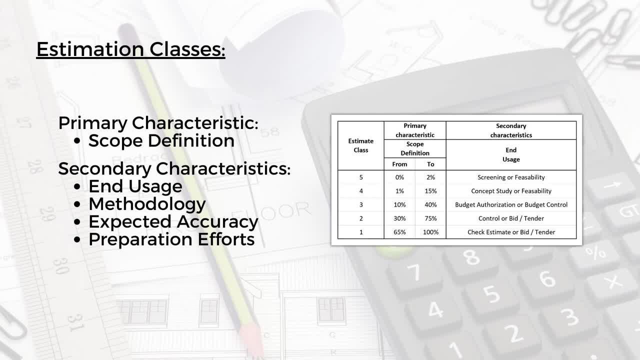 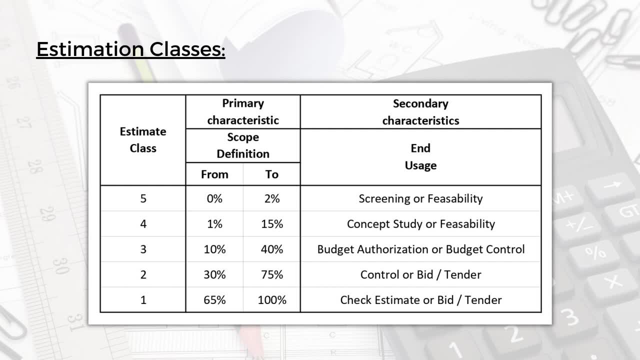 use and the methodology and the expected accuracy and the efforts required for the preparation. So when we take a closer look here, we have the estimate class. So when we are talking about class five, the scope definition will be between zero percent to two percent. So we don't have the scope. 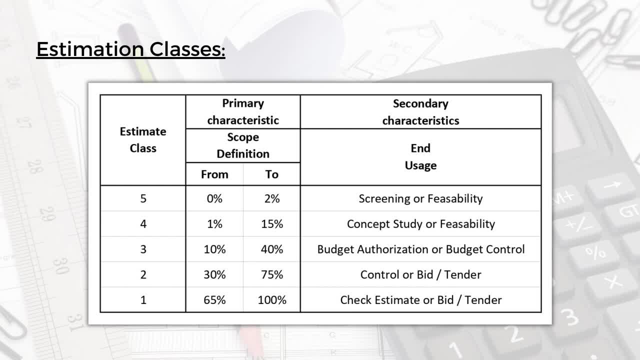 defined yet And this class can be used for screening or feasibility as an ND usage, which is a secondary characteristic. Class four, for example, the scope definition will be between one percent to fifteen percent And this class can be used for concept study or feasibility. And the class three, the scope definition will be